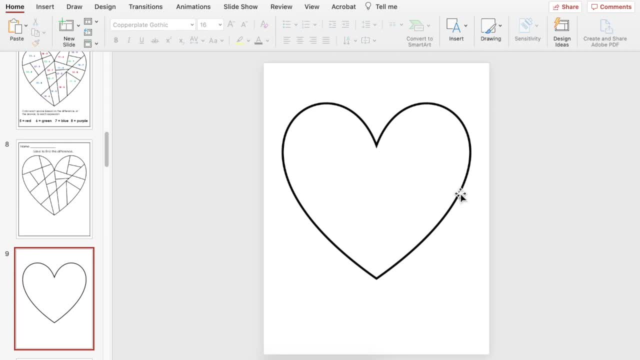 to color. it's not really related to math. or if you wanted to use geometric shapes for your students to color, more so in the primary grades, you can just insert your shape, make it large, and there's a coloring sheet for them To break it apart with the lines I'm going to go back to. 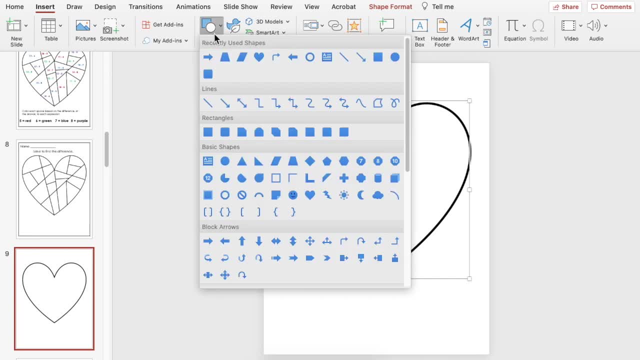 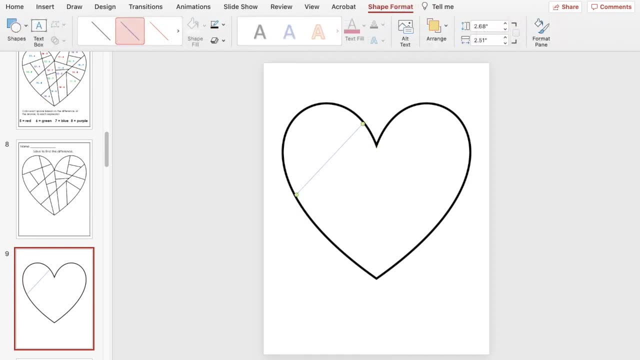 insert, go back to shapes and then select line and just draw lines going across the heart, And I'm going to get up closer to make sure the lines are reaching the edges, And we're going to change that line color to black and the weight let's do about 3.. 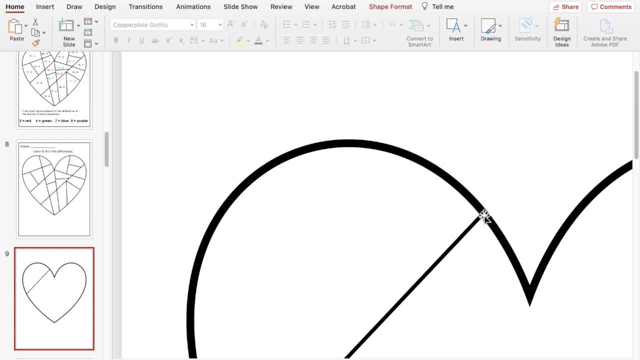 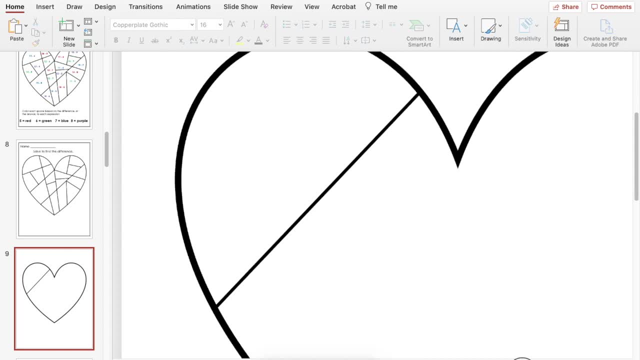 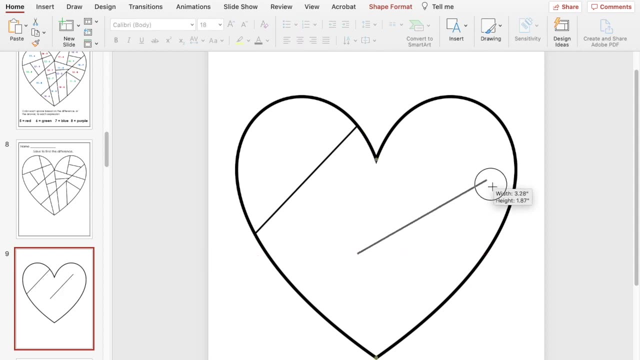 So let's go to the top and make sure it's touching the edge. so there's no space and there is our first line. So we're going to zoom back out and I'm going to just duplicate that line and put it in a different spot, duplicate it again. All I'm doing is duplicating. 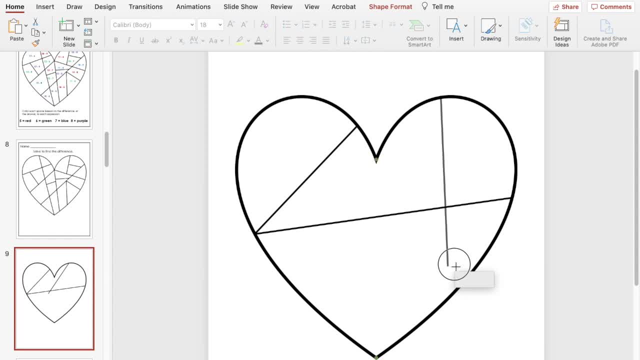 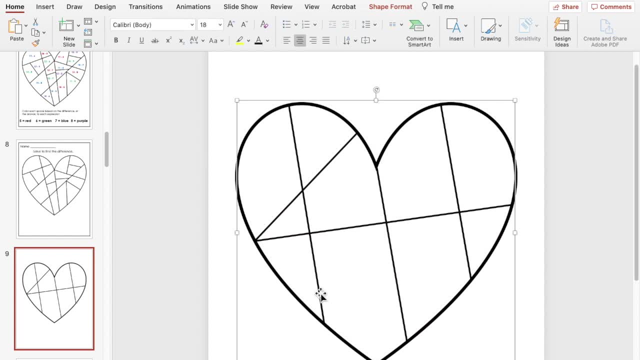 my lines and changing it, changing the direction and where it goes on the heart. You can also make smaller lines. You want to take your line and shrink it because you don't want it to be that long. You can do that. It all depends on how many separated areas that you. 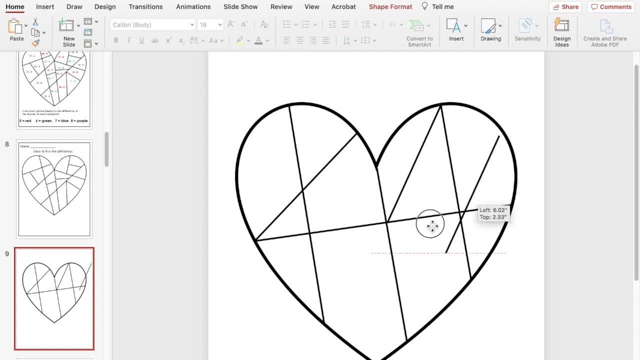 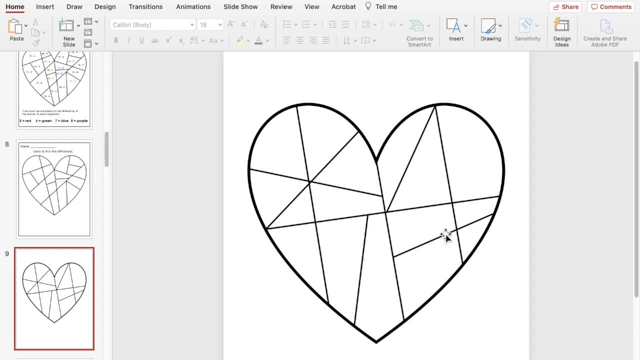 want and if you're going to include math problems, how many math problems you want. if you want a specific number, All right, so I'm going to count: 1, 2, 3, 4,, 5,, 6,, 7,, 8,, 9,, 10,, 11,. 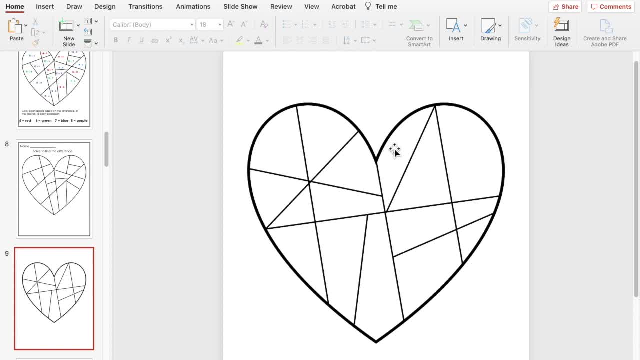 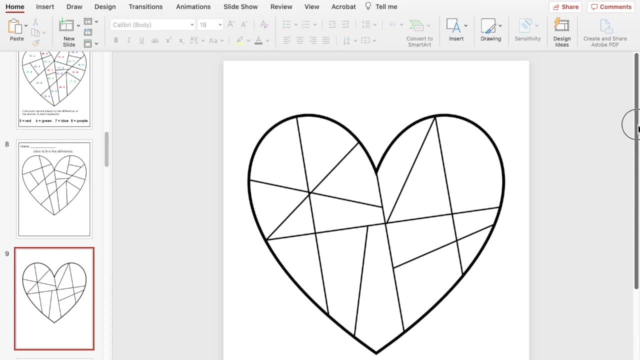 12,, 13,, 14,, 15,, 16.. So if I wanted to create problems, I can have four sets of different types of problems. So that looks good. So now what I want to do is create the directions for how to solve their problems. So again you. 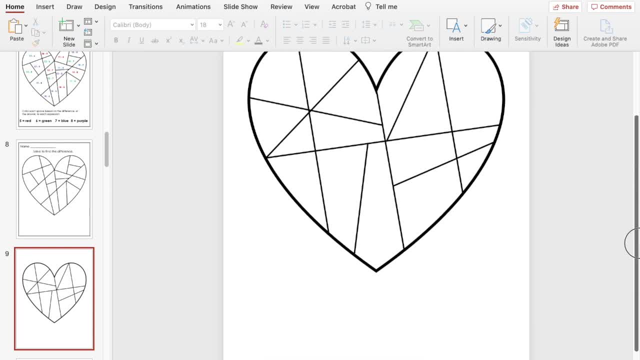 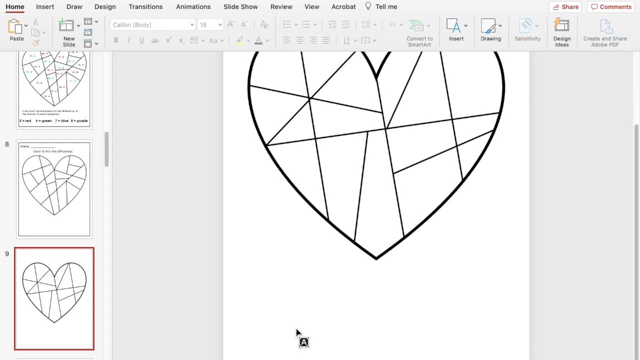 can stop here with a coloring page with different parts and give the students the freedom to color it how they want, but we're going to add in math problems, So I'm going to create a text box and I want this to be subtraction. So I want them to find the difference and 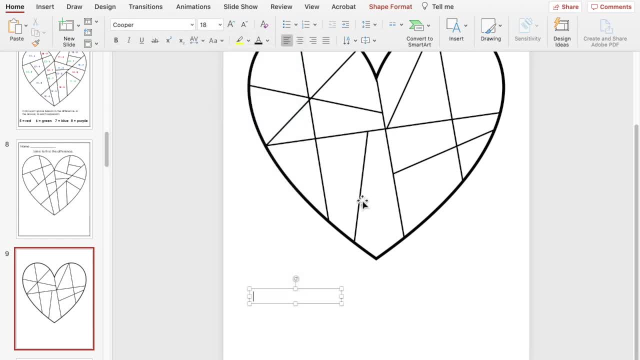 I'm going to give them the answer and they're going to color based on that answer. So if the answer is 5, that means they are going to color it red. color the space red. If the answer is 6, they're going to color it green. 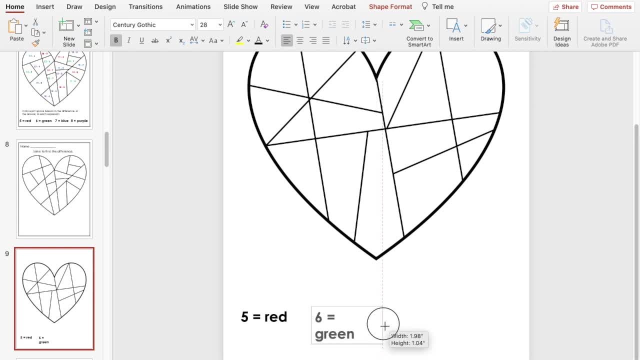 I'm going to do one for 7, and one for 8.. So now we're going to go in and write the problems. So I'm here in math and I don't. and you want to make sure they're spread out based on the colors that you chose. 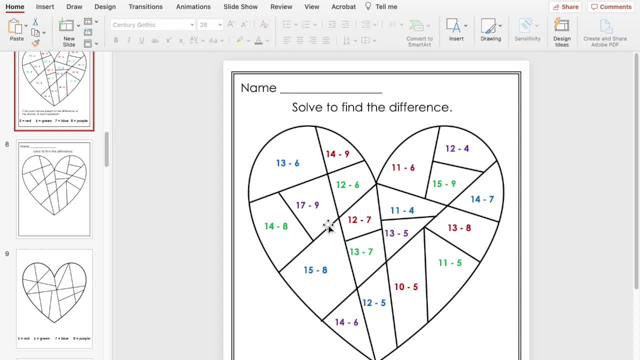 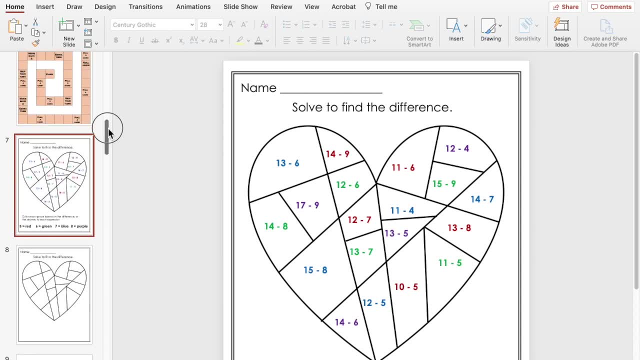 okay. so it's gonna look like this when we're done, because we want to see how the colors are going to be spread out across the heart. but that's not what you're going to show the students. you're gonna have basic black or the problems in one color, probably black or gray, so that they don't know ahead of time which. 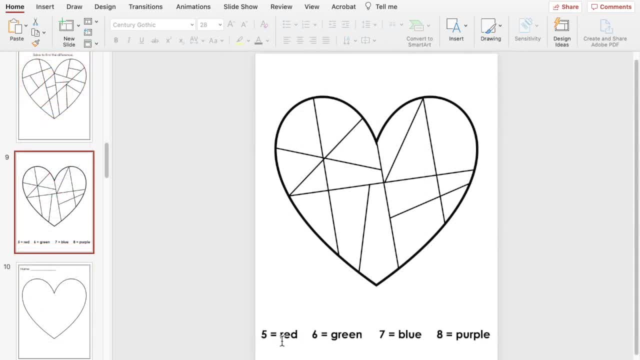 colors are gonna shade in the heart, so I'm gonna start with red and I want these problems not to be that hard, so I'm going to duplicate and do: let's change it to red and we're going to make the problems like a two-digit by minus a. 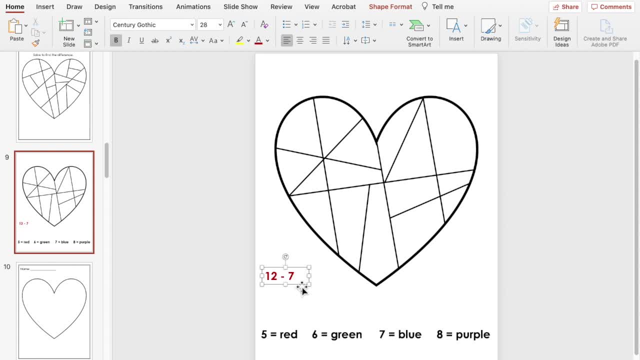 one-digit number two. twelve minus seven, that's gonna equal five. so I'm gonna put that there and I'm actually going to go to the smallest space and make sure that the item can fit. so they can't fit. I need to make it smaller, but instead of making it, 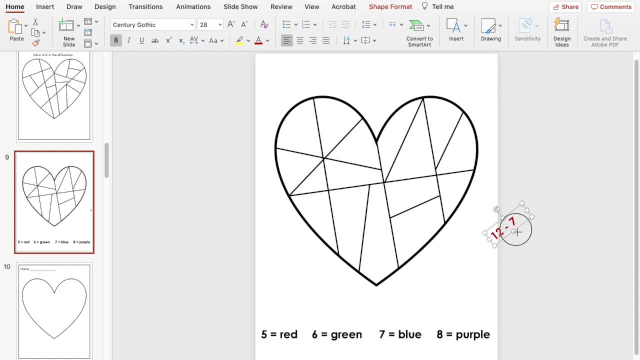 small. I'm actually gonna move. so again, let's look for the smallest space here so that fits. so twelve minus seven. so I'm gonna do another one here and let's do 11 minus 6 and then duplicate that again. let's do one up here.